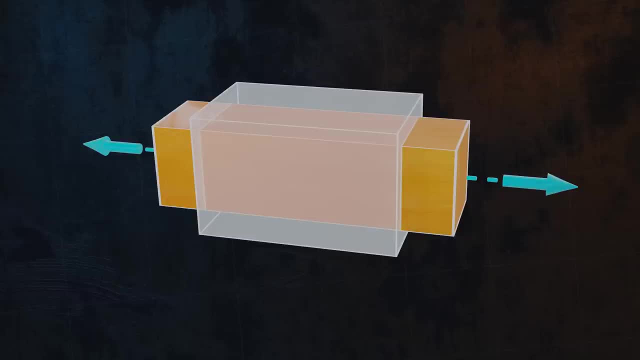 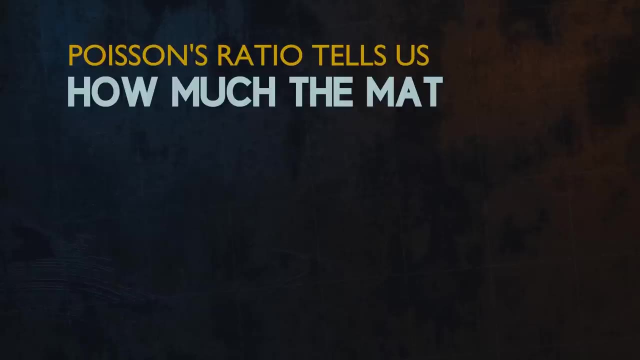 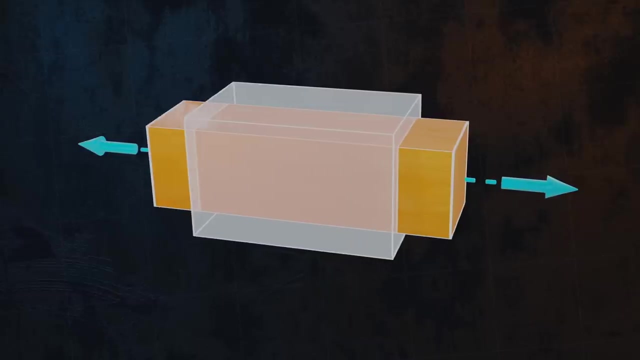 concept here is that when you apply a load to a material in one direction, the material will also deform in the lateral directions. Poisson's ratio is the parameter that tells us how much the material will deform in the lateral directions. To define Poisson's ratio more precisely, 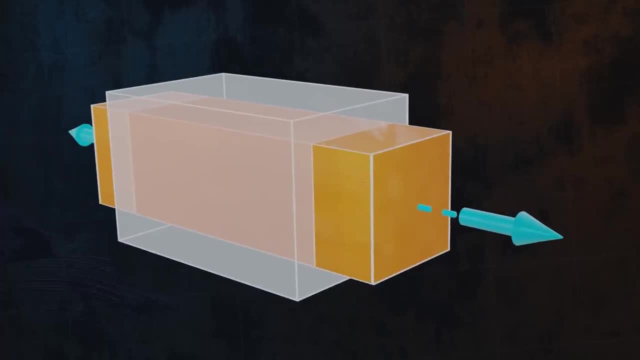 let's take a closer look at the case where a tensile force is applied. First, let's give names to the various parameters involved. Lx, Ly and Lz are the original dimensions of our cuboid along the x, y and z axes. 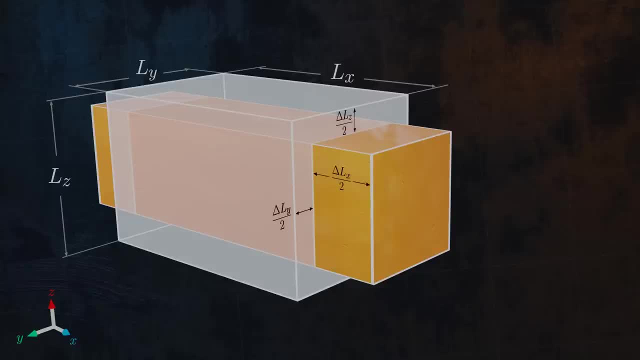 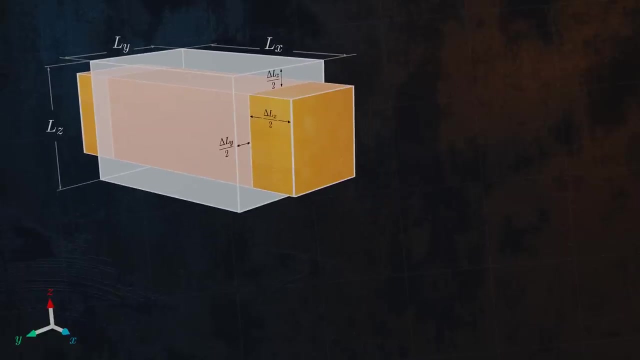 Delta Lx, Delta Ly and Delta Lz are the changes in these dimensions after the load has been applied. They are shown as being divided by two, because the change in dimension occurs on both sides of the object. Next, we can write out the strains in all three directions As a quick reminder. 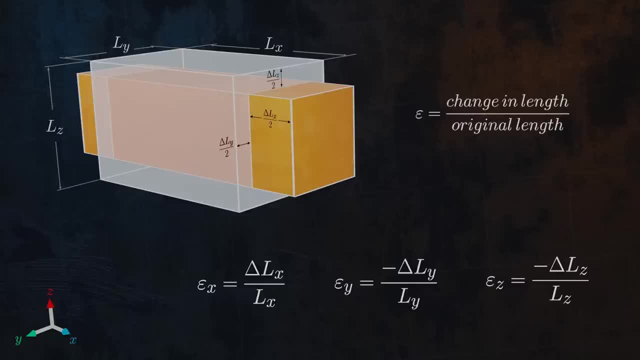 strain is a measure of deformation and is defined as the change in length divided by the original length. It is denoted using the Greek letter epsilon and is usually expressed as a percentage. When we apply our longitudinal load, it turns out that the resulting strains in 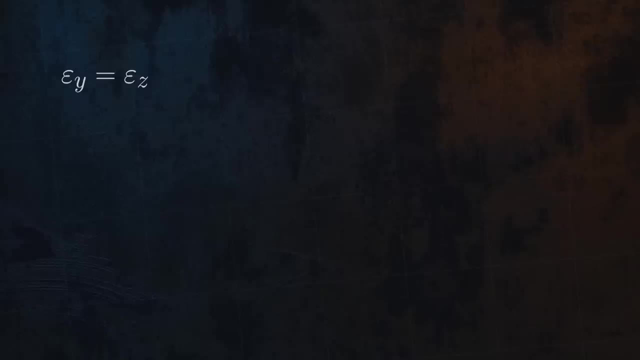 the lateral directions are equal, And here is the interesting part- They are proportional to the strain in the longitudinal direction. The ratio between the longitudinal strain and the lateral strain is actually a material constant. You might have guessed it by now, but we denote this material constant with the Greek letter ν and we call it Poisson's ratio. 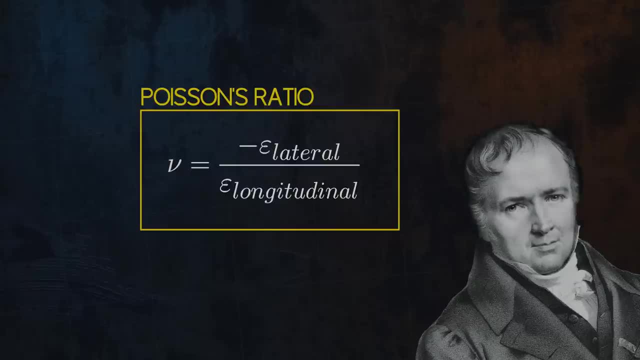 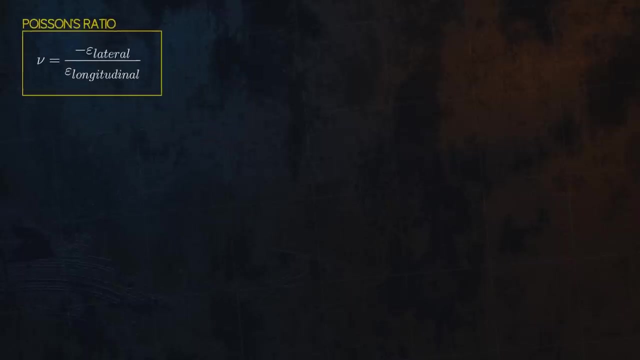 By the way, Poisson's ratio is named after this guy, Simeon Dornier Poisson, the famous French mathematician who formally defined the ratio in a note published in 1827.. You might be wondering why a minus sign slipped into the equation. Remember that by convention. 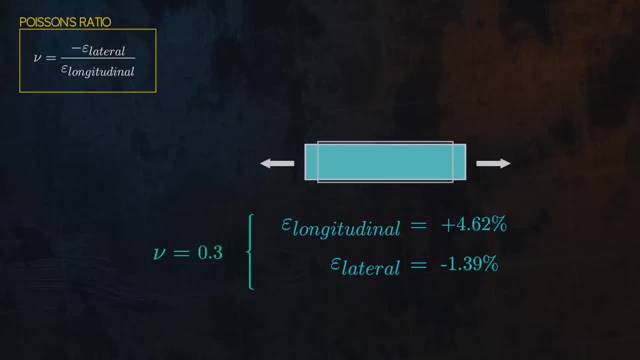 tensile strains are positive and compressive strains are negative, The minus sign is just there, so that for the typical case where the lateral strains are opposite in sign to the longitudinal strains, we get a positive sign. Now is probably a good time to mention that this equation and the concepts described in this video. 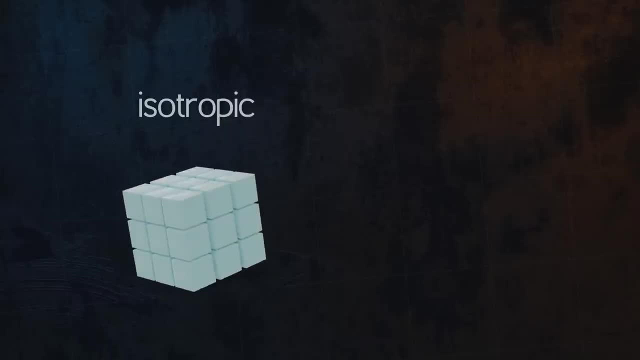 only apply for isotropic materials, which are materials which have the same properties in all directions. We are also assuming that the materials are deforming within the elastic region. Things get a bit more complicated when plastic deformation is involved. Anyway, to summarize, Poisson's ratio is a dimensionless material property. 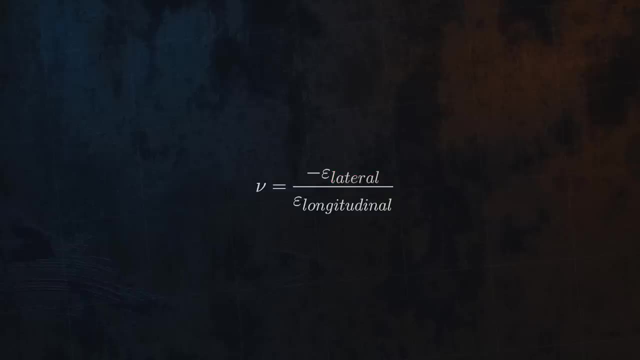 which tells us how much a given material will contract in the lateral direction. In other words, when we pull on it, it will contract in a longitudinal direction. Now that we know what Poisson's ratio is, we can look at some typical values for different 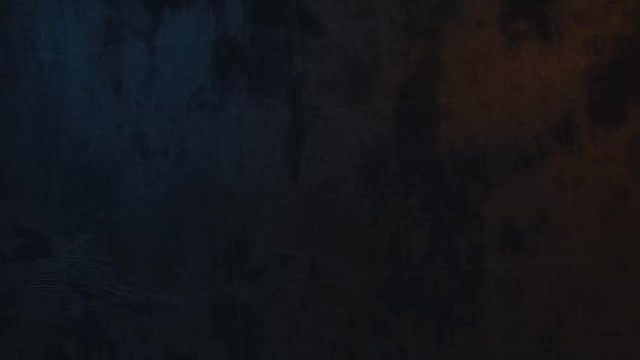 materials. Without getting too deep into the math behind it, it's useful to know that the theoretical range of possible values for Poisson's ratio goes from negative one to point five. In practice, most real materials have a Poisson's ratio of somewhere between zero and point five. 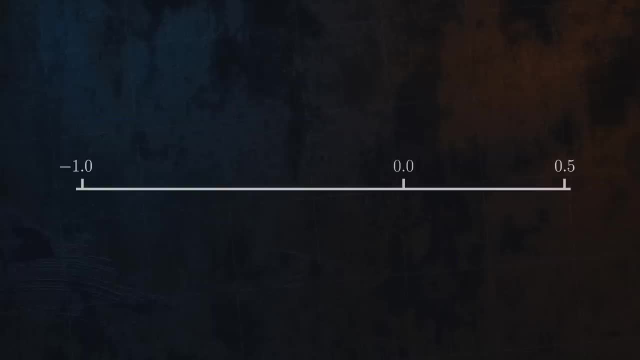 Here are some typical values for a few selected materials. Now let's look at how different values of Poisson's ratio affect how a material deforms under loading. We'll keep things simple and consider a two-dimensional case. Most materials have Poisson's ratios between zero and point five When a tensile force is applied. 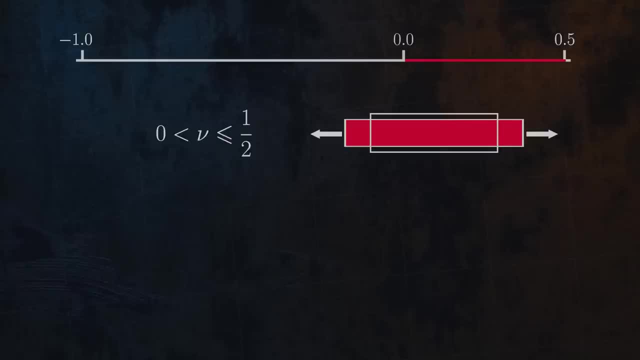 these materials contract in lateral directions, as we have already seen with our orange cuboid. Materials with a Poisson's ratio of zero are interesting. When a longitudinal tensile force is applied, there is no deformation in the lateral directions. One material that behaves in this way: 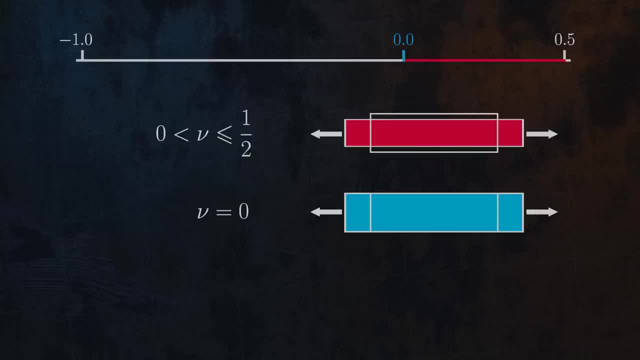 is cork, which has Poisson's ratio close to zero. This property makes it a very useful material for certain applications. A great example is the cork in a bottle of vodka Wine, Because it doesn't expand laterally when compressed, as you can see here. 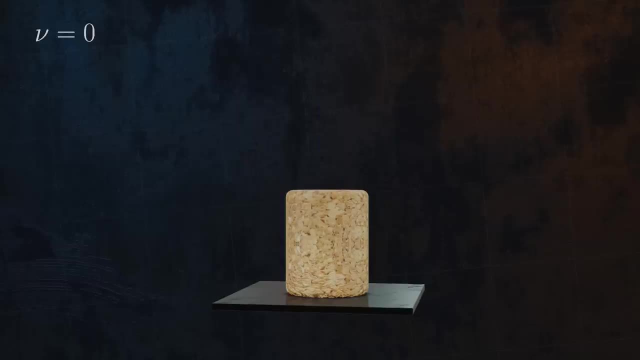 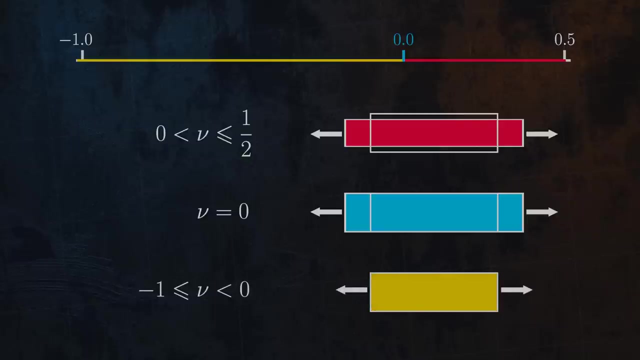 it can easily be inserted into the neck of a bottle. A material with a larger Poisson's ratio would be much more difficult to insert as it would expand in the lateral directions when compressed. Finally, we have materials with negative Poisson's ratios. These are known as 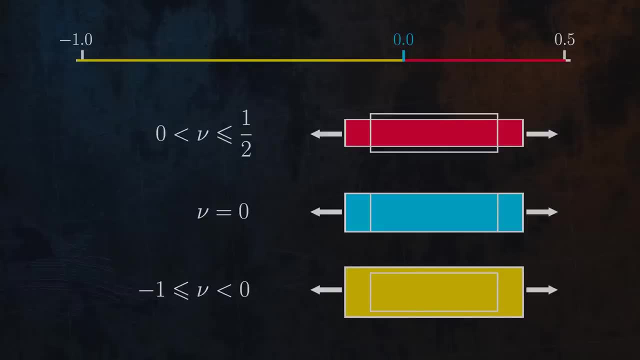 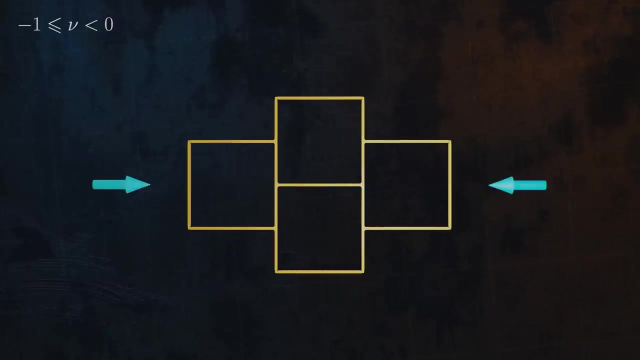 auxetic materials. They expand laterally when pulled and contract laterally when compressed, which seems counterintuitive. These are mostly engineered materials, like special foams, rather than materials occurring naturally in nature. This animation should give you an idea of how it is possible to get negative. 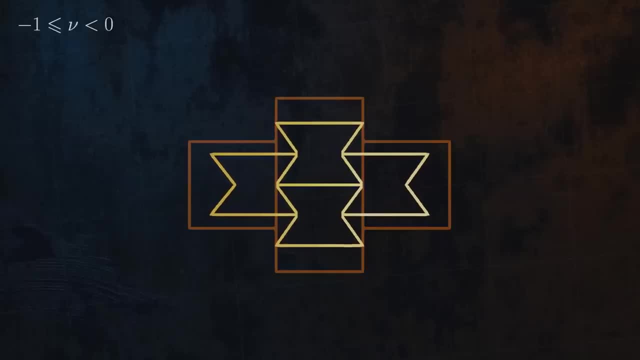 Poisson's ratios. You can see that as the material is compressed, both its longitudinal and lateral dimensions are reduced. For a typical material with a Poisson's ratio larger than zero, you would expect the lateral dimensions to increase when the material is compressed. 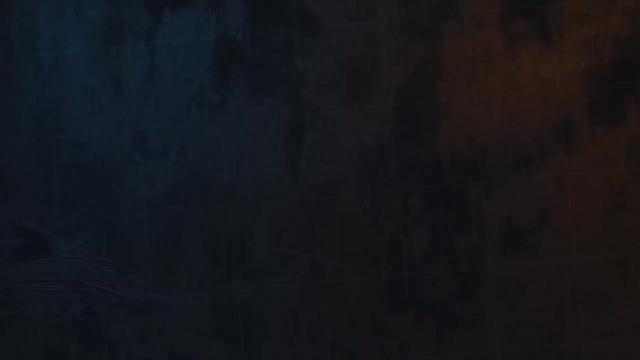 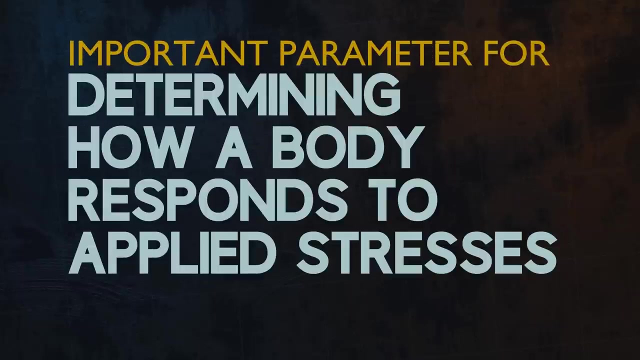 Because it tells us how a material deforms. Poisson's ratio is a very important parameter in continuum mechanics for determining how a body responds to applied stresses. Let's look at a simple case of uniaxial stress: the tensile test. 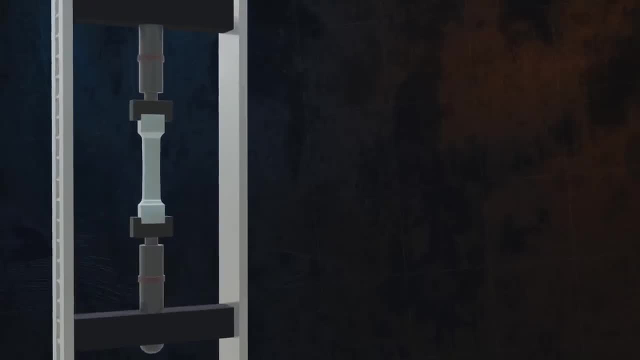 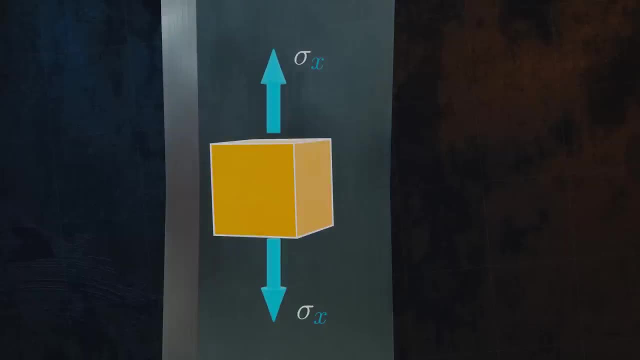 It is easy enough to determine the strains acting on a small piece of the specimen under test. The applied stress is a normal stress in the x-direction sigma x. The strain in the longitudinal x-direction is simply given by Hooke's law as sigma x divided by the Young's modulus e. 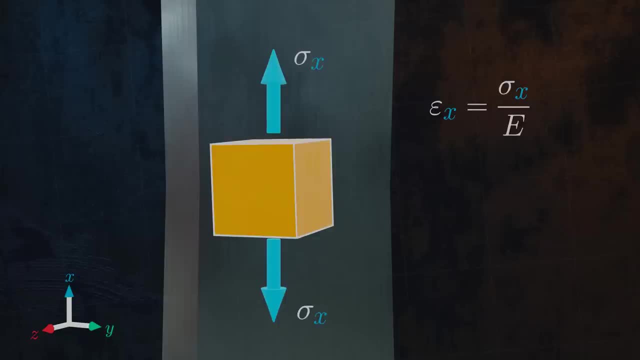 Hence the仔est path runs in the lateral, y- and z-directions. Even though there are no stresses acting in the lateral y and z-directions, there will be strains in these directions as the material will contract laterally. The strains in the lateral directions are obtained by multiplying the longitudinal strain. 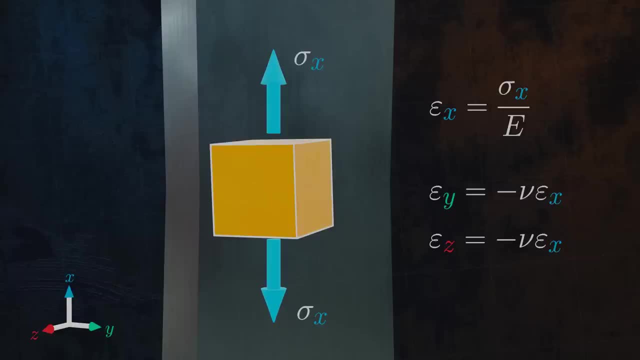 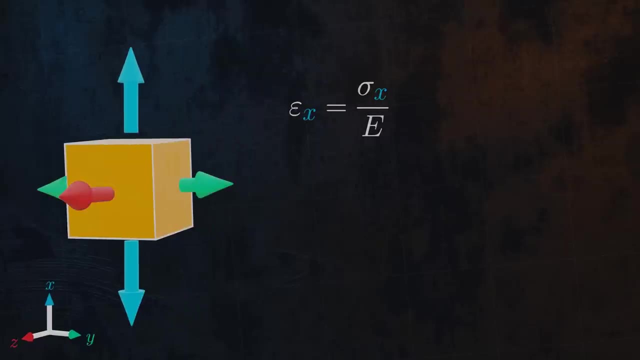 by Poisson's ratio. This is just using the definition of Poisson's ratio which we covered earlier. But what if we look at a more complex case where we have triaxial stress with different case? we can't just use Hooke's law to determine the strain in the x-direction. 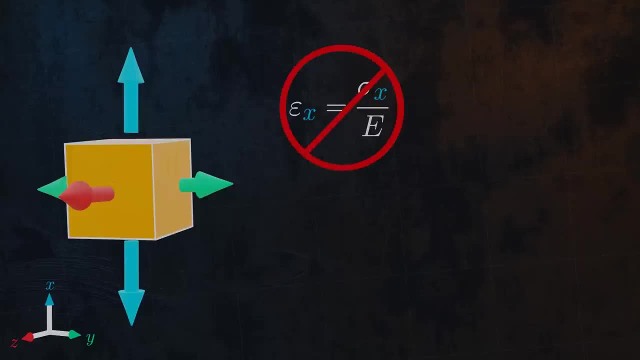 because it will also be affected by the strains in the y and z directions. The simple version of Hooke's law for uniaxial stress no longer applies, because the strains in one direction will depend on the stresses applied in all three directions. We can use Hooke's law in combination with the equation for